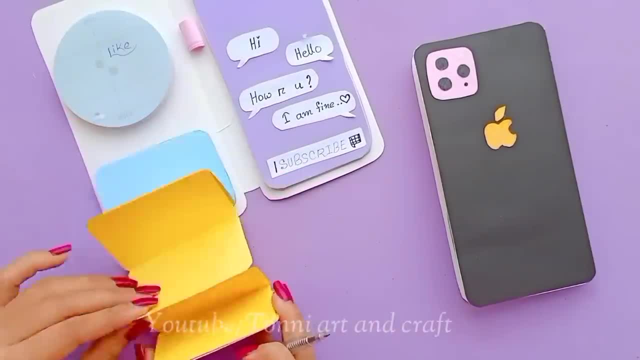 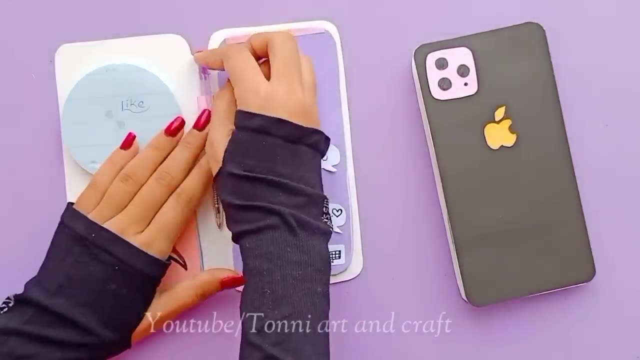 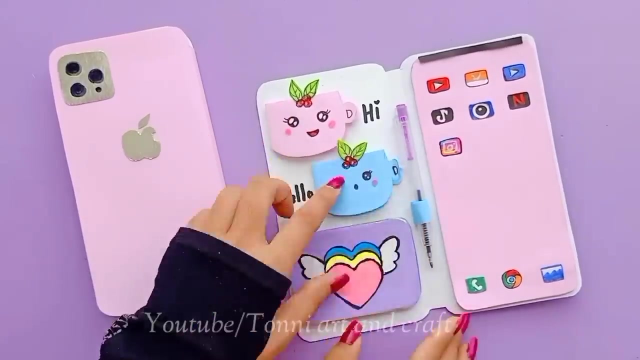 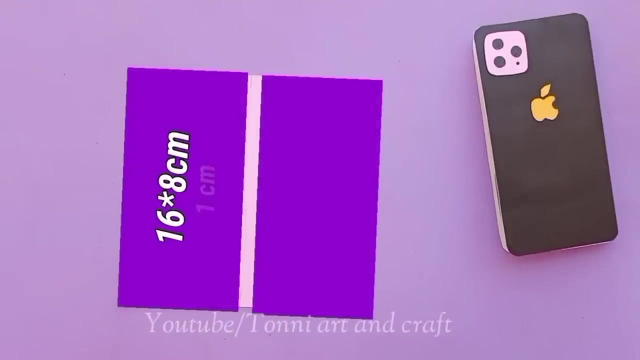 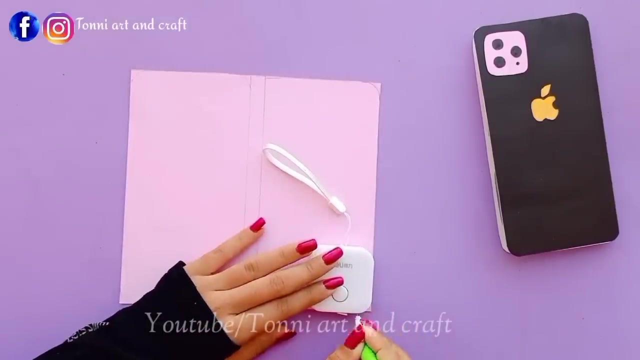 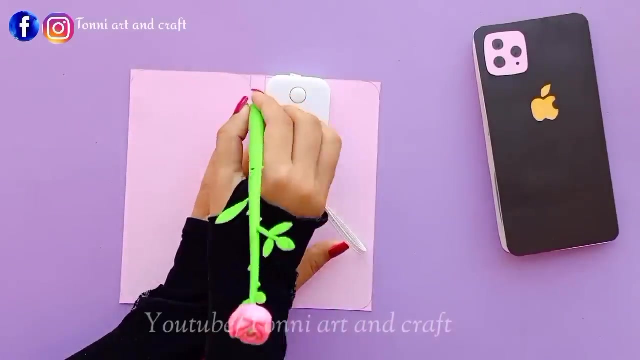 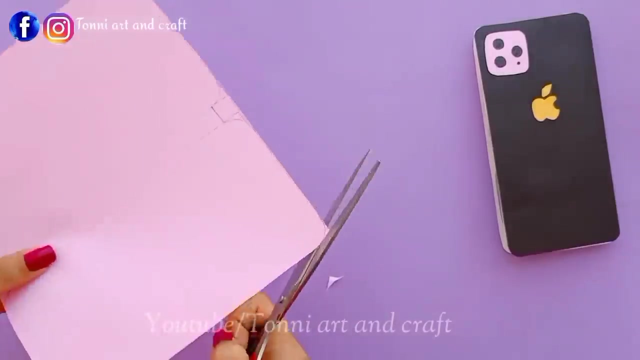 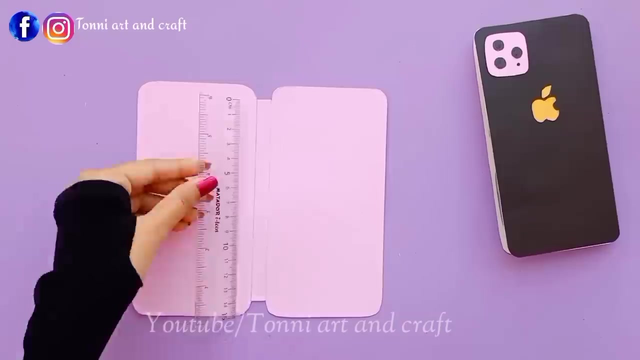 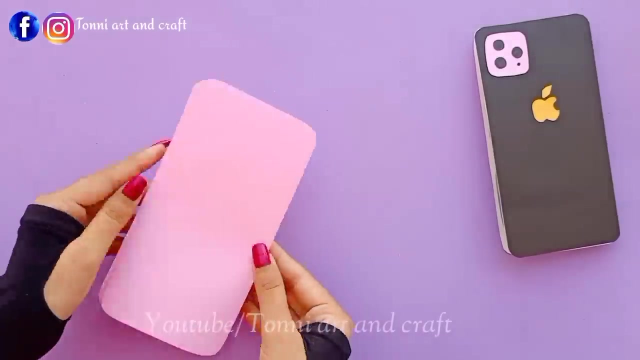 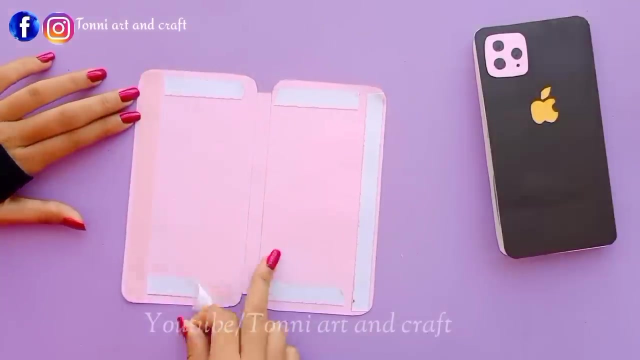 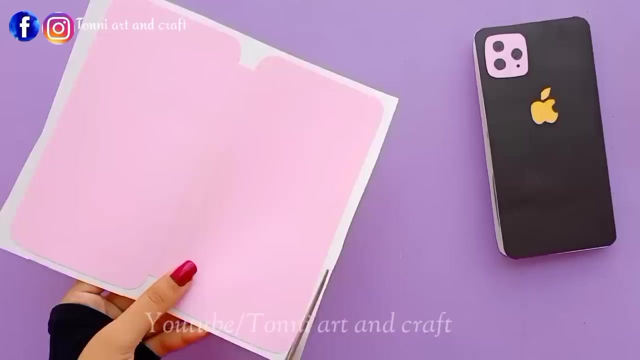 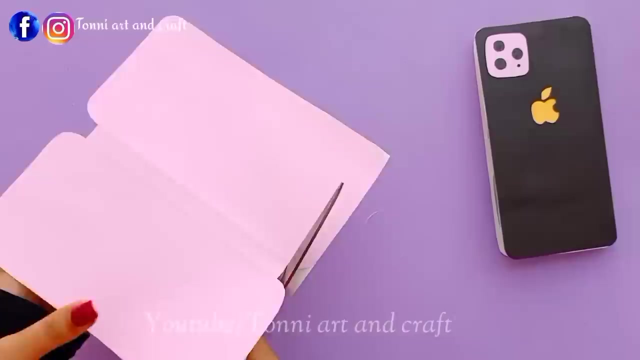 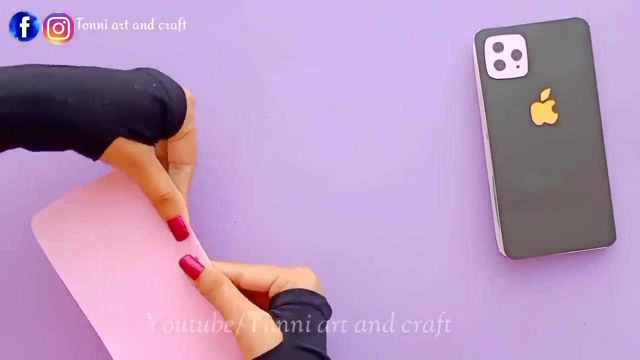 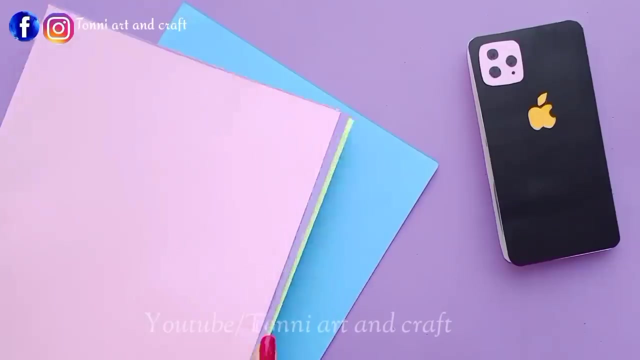 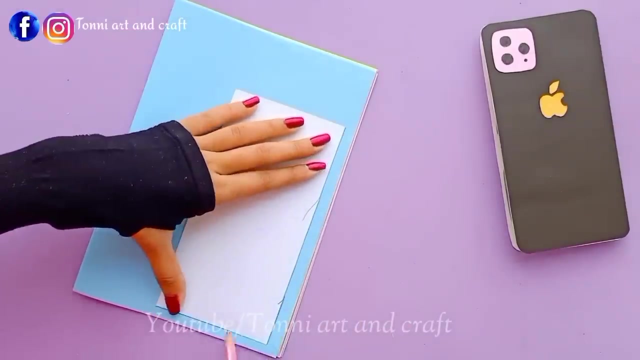 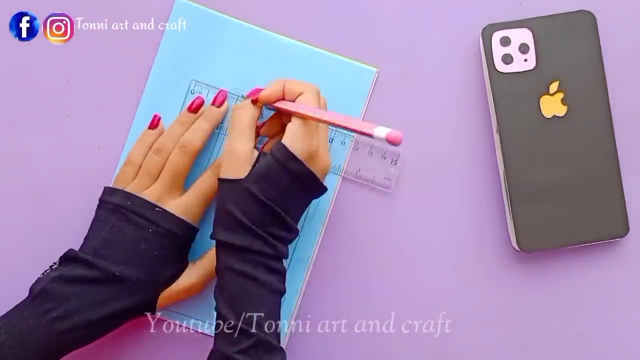 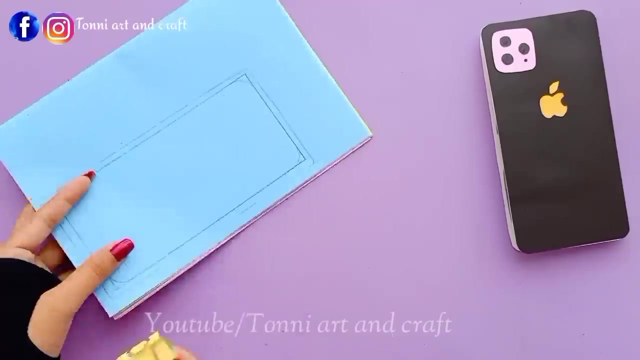 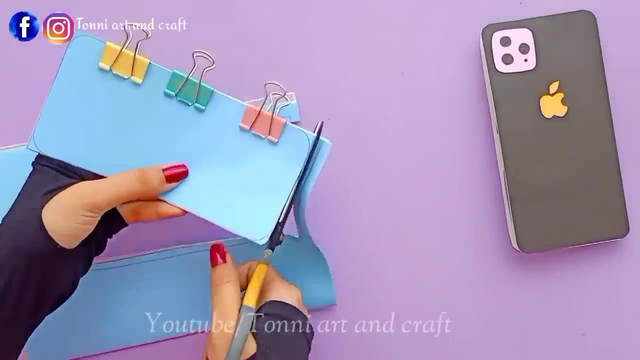 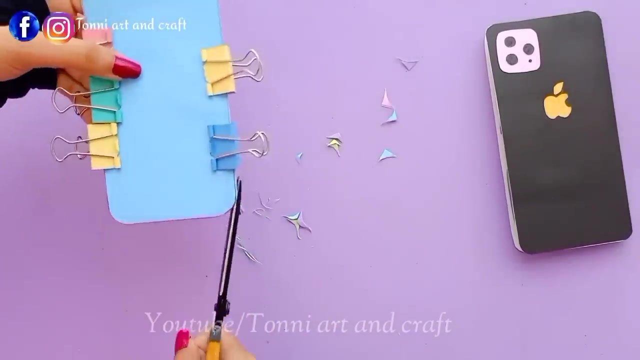 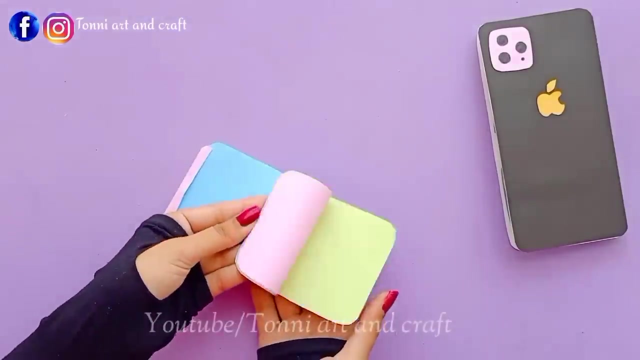 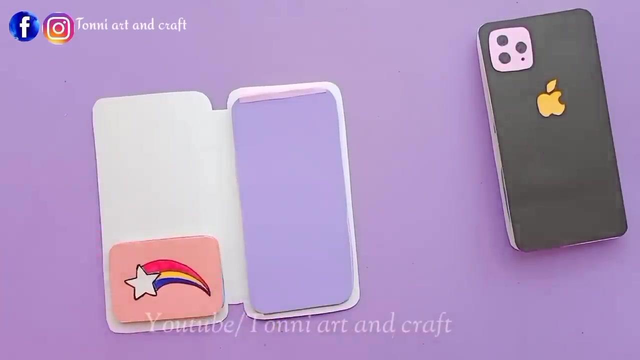 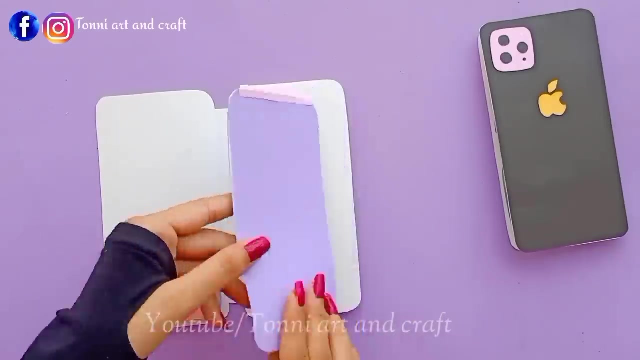 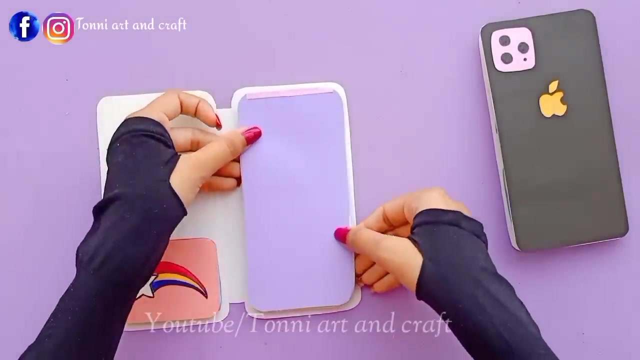 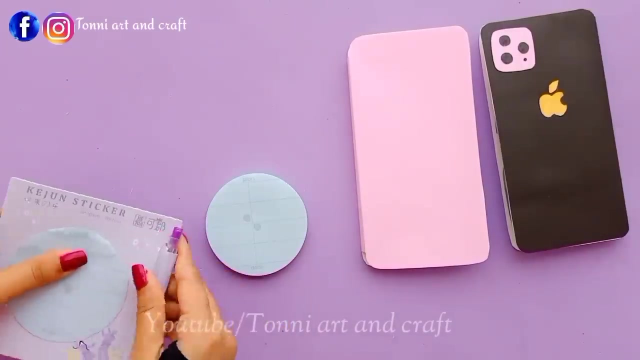 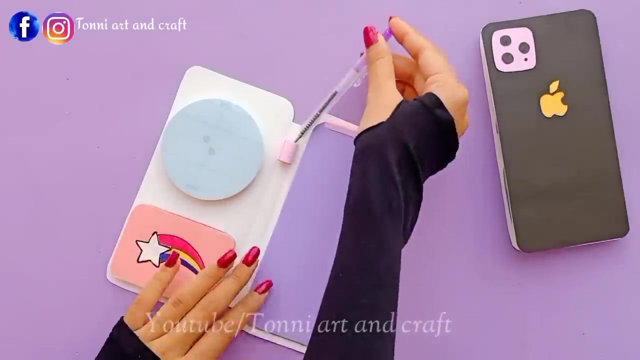 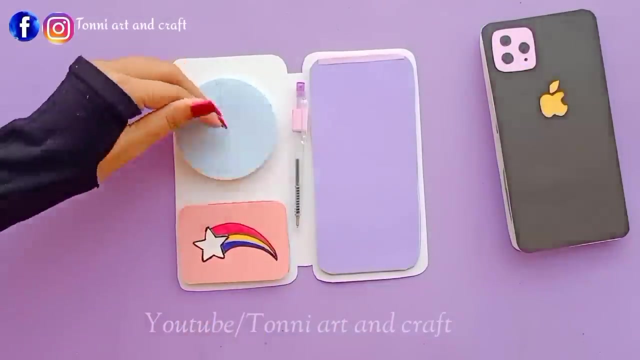 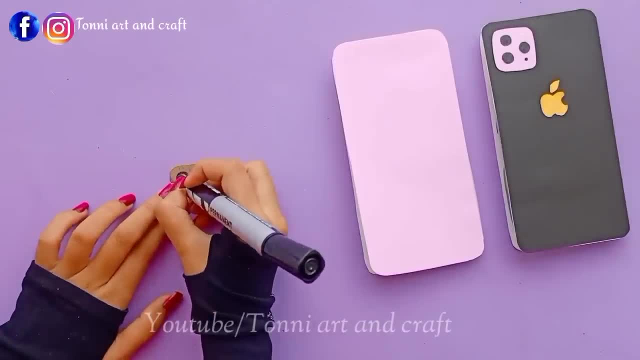 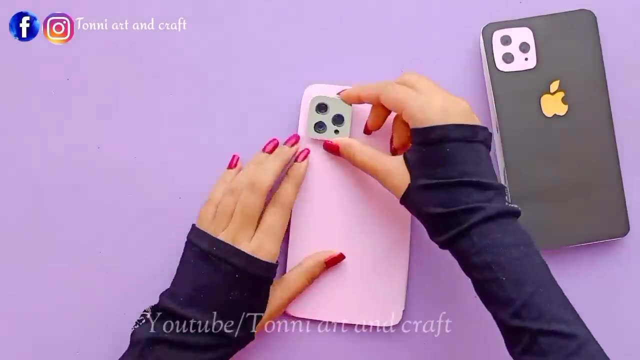 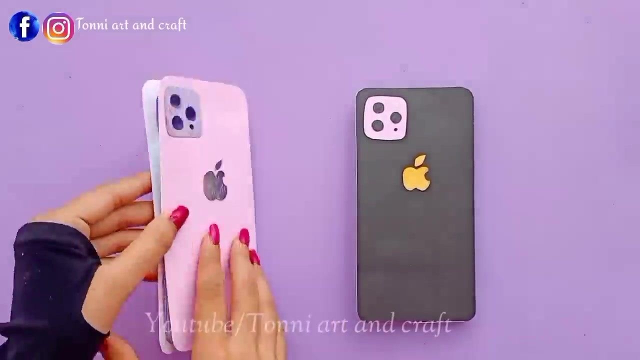 Easy come, easy go. No stress, I'm good without it. Easy come, easy go. Let's keep it fun and simple. Easy come, easy go. I've been looking for answers something more, Holding the past in my hands. 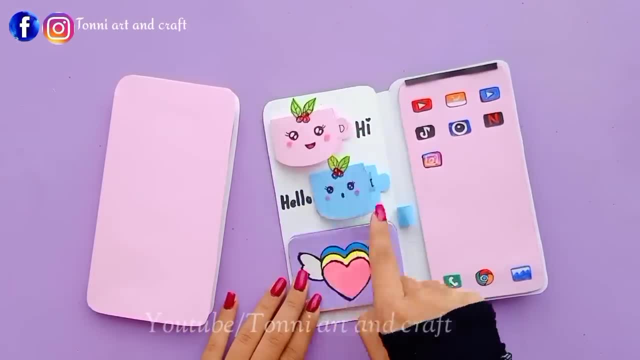 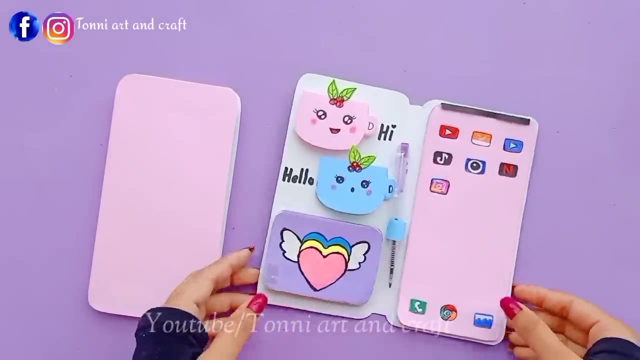 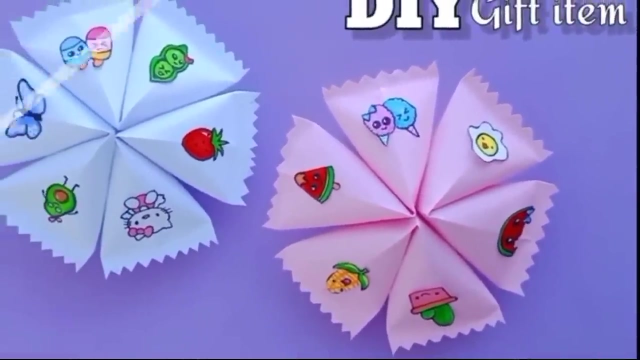 Now I'm fighting for someone I've ignored To find who I am, And I've been begging All the time. I need to get back to me And I'm missing all the ways that you and I used to be, And I'm putting the fire to the floor. 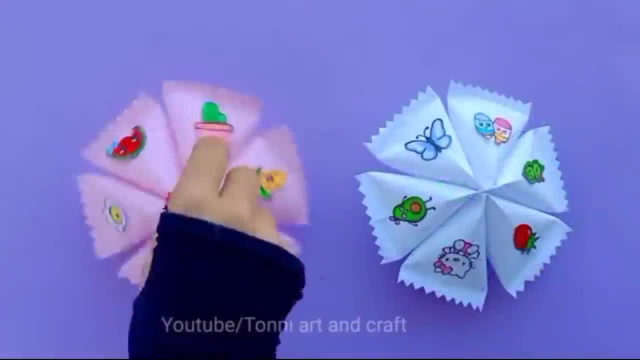 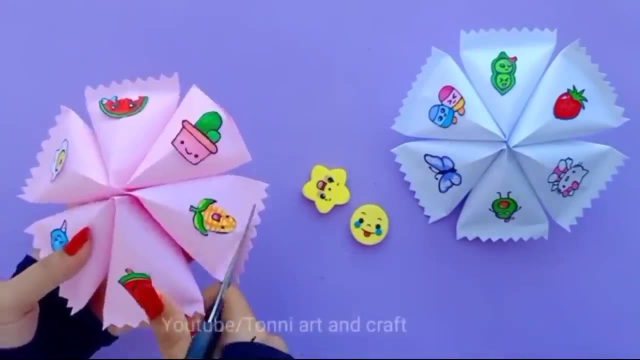 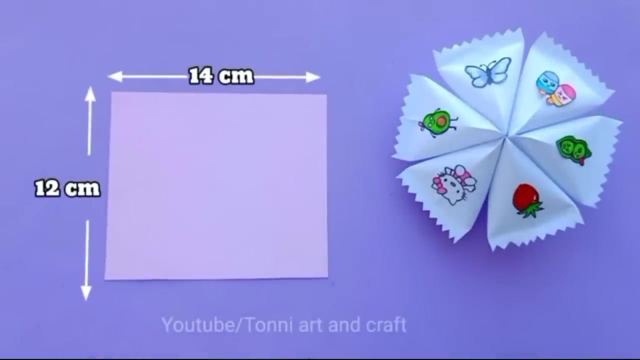 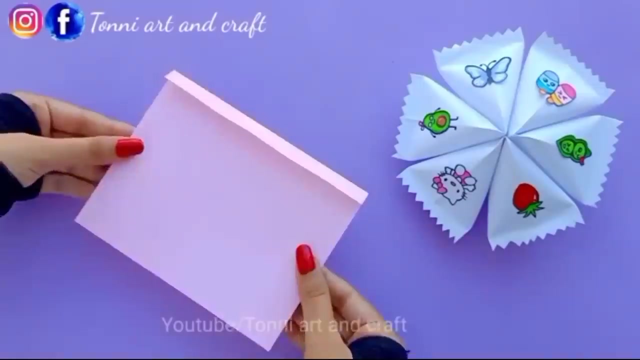 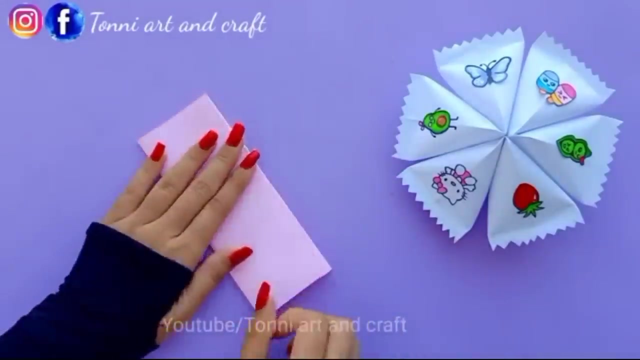 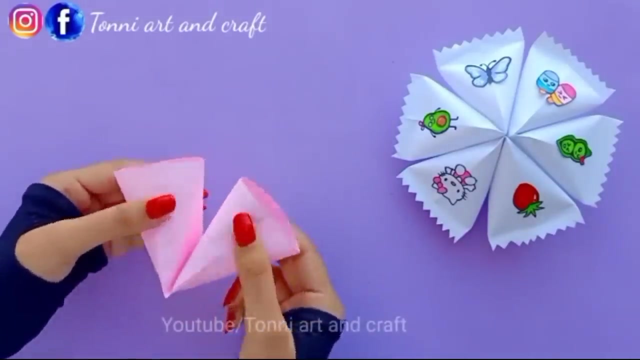 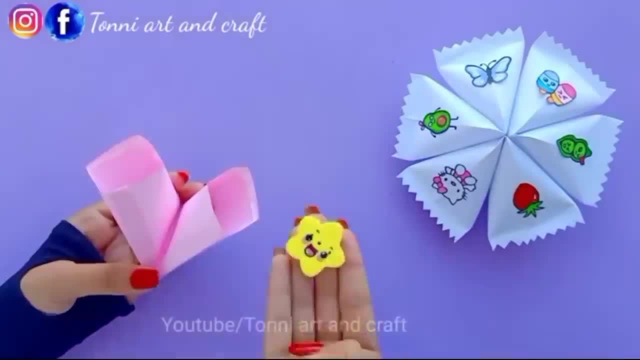 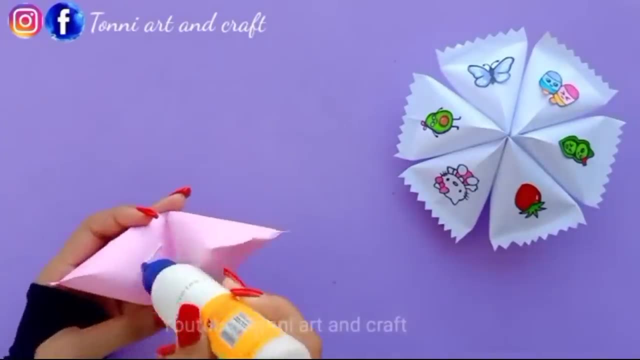 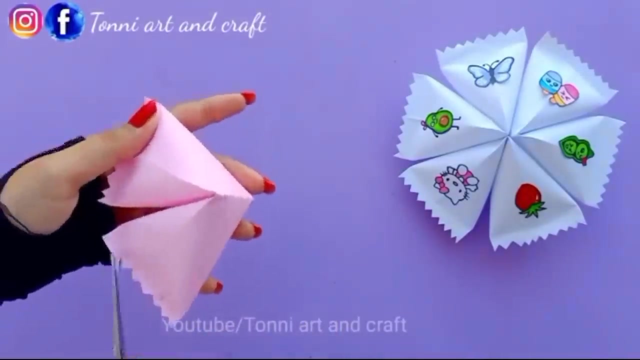 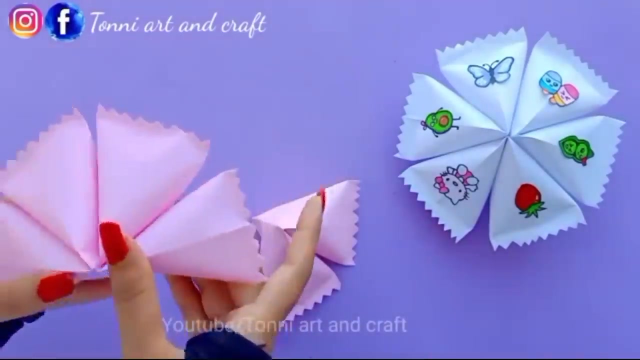 You've been fighting a war I cannot win, Walking the world all alone, And I'm finally finding what's within, Now that I know, Cause I've been busy. I've been chasing waterfalls, I stopped believing in some kind of miracle And I've been staring at the sun for too damn long. 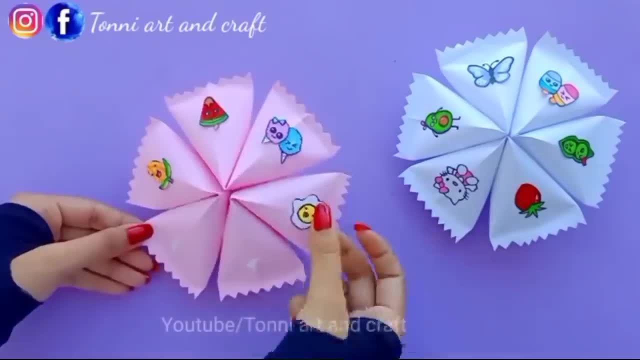 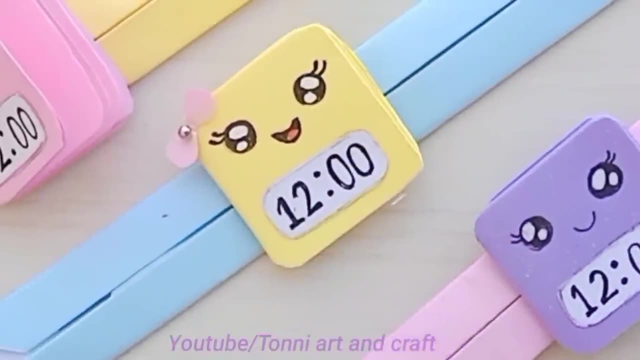 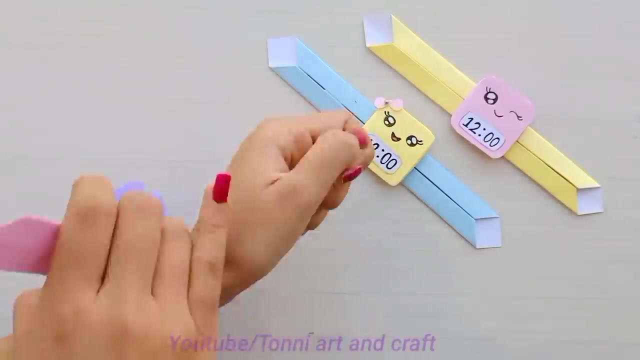 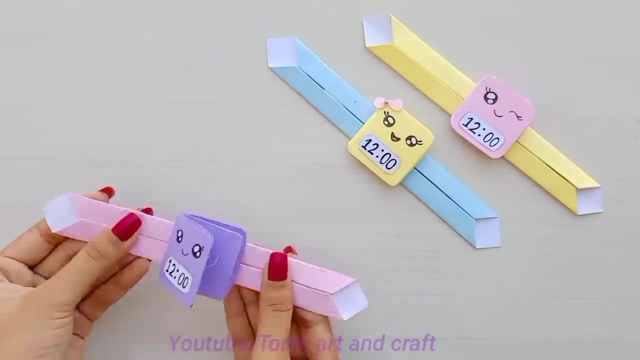 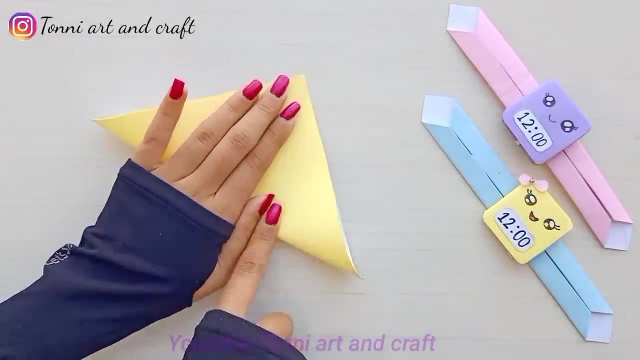 But when I opened up the door, he let me back to You, you, you, you. Then I opened up the door, he let me back to You, you, you, you. Then I opened up the door, he let me back to. 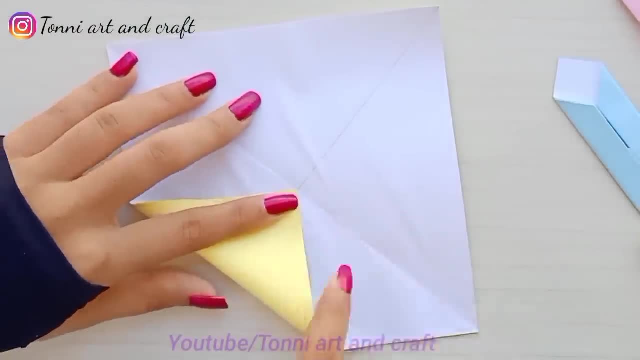 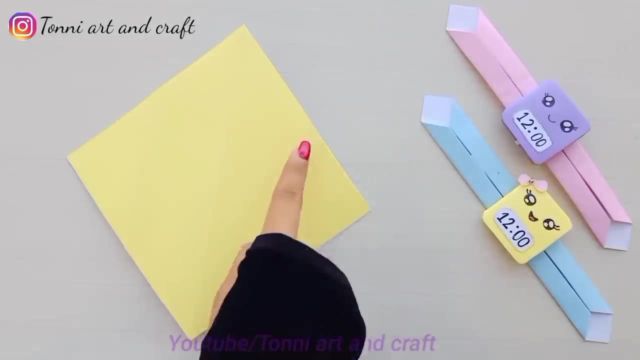 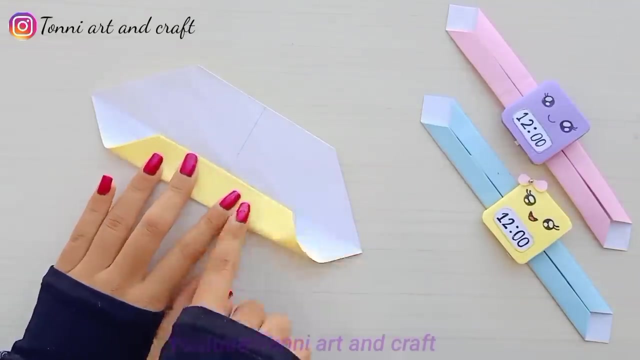 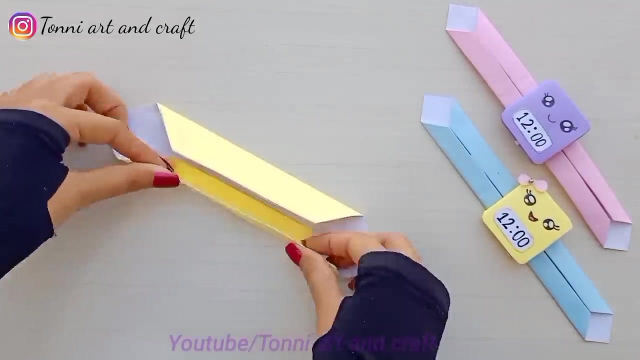 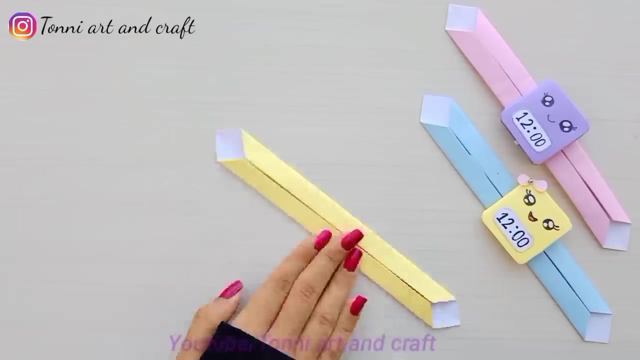 Oh, I've been thinking of you every weekend. Tell me you too. tell me you too, Don't you feel you miss me and you wanna kiss me? I feel it too, baby. I feel it too. Come around to me. I will hide that. you stay close to me all the night, like 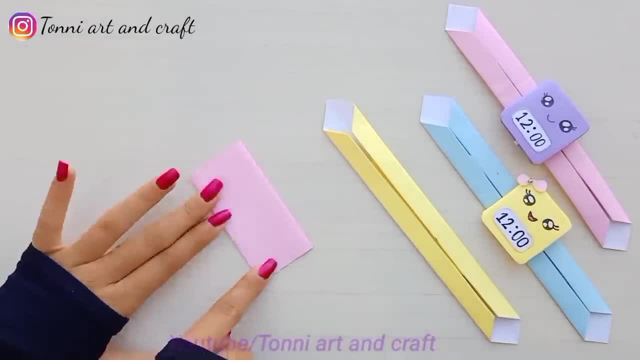 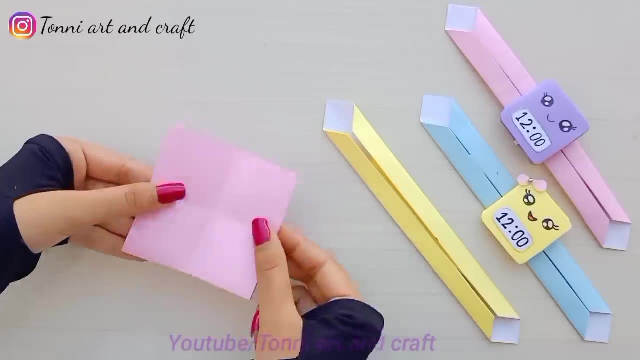 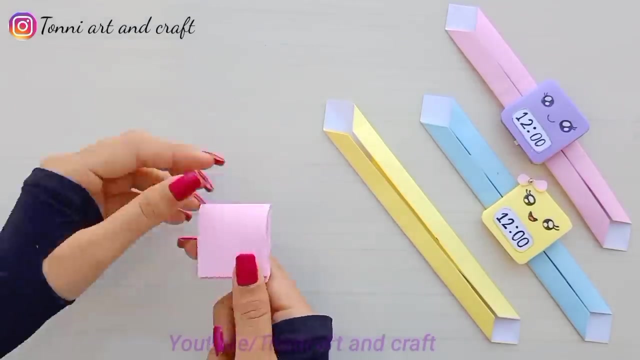 Ooh, yeah, yeah, ooh, yeah, yeah. Come around to me. I will hide that. you stay close to me all the night like Ooh, yeah, yeah, ooh, oh. I've been thinking of you ever again. 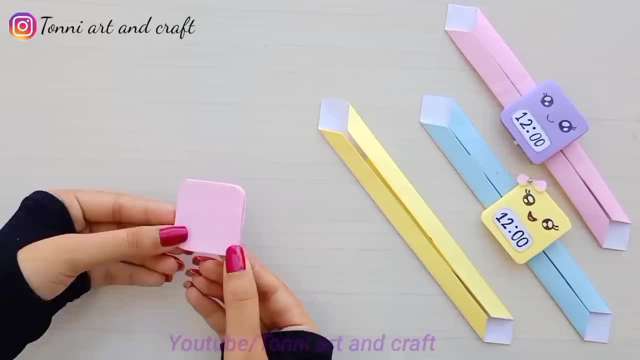 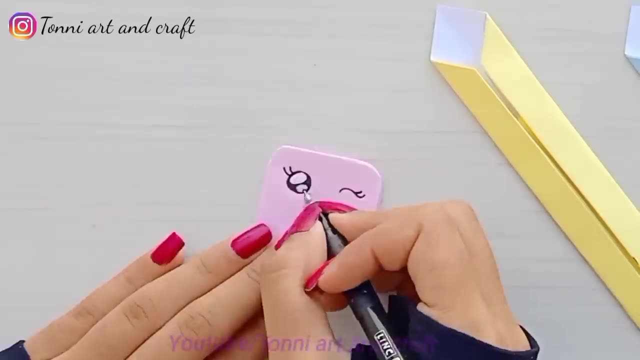 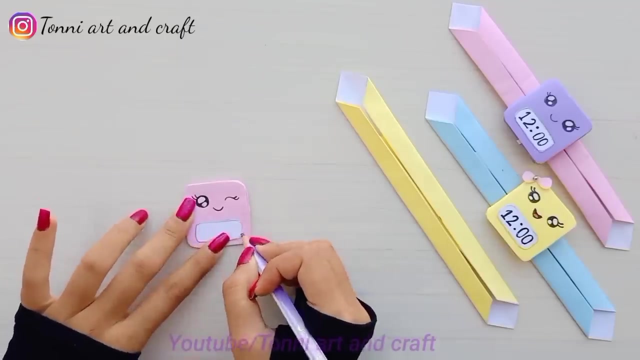 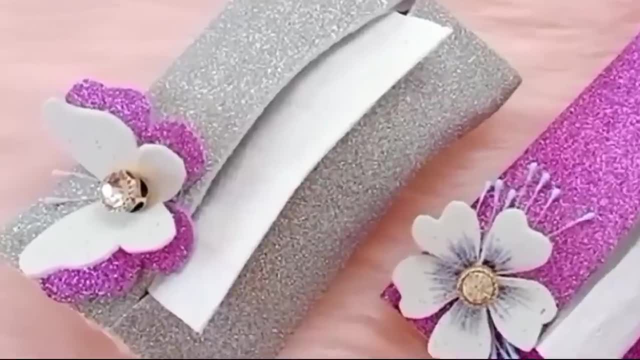 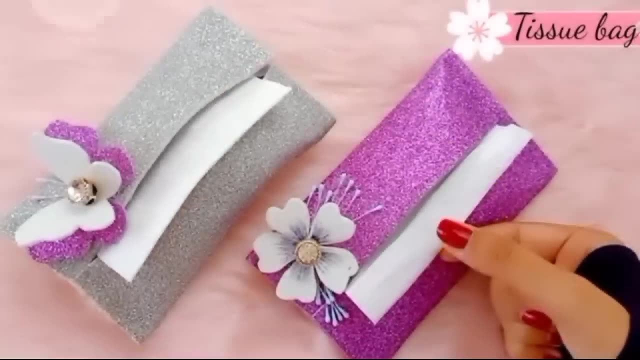 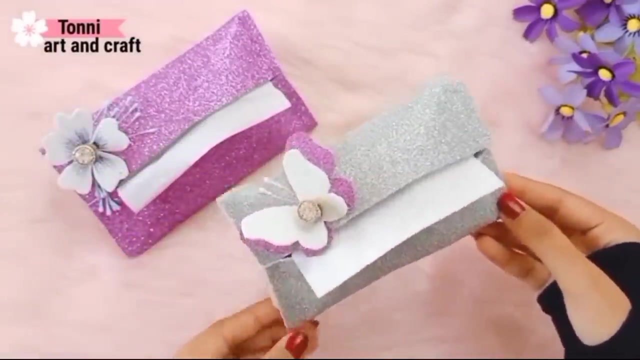 Baby, don't you feel it too. tell me, baby, don't you feel it too? Ooh, I've been thinking of you ever again. Tell me, you do. tell me, you do. Don't you feel you miss me and you wanna kiss me? 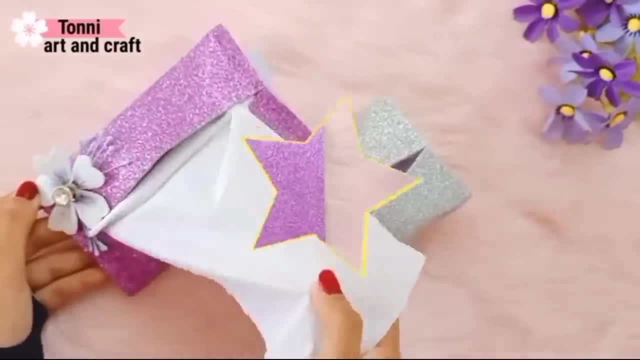 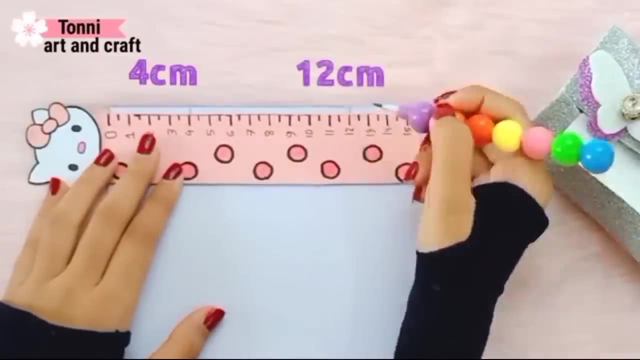 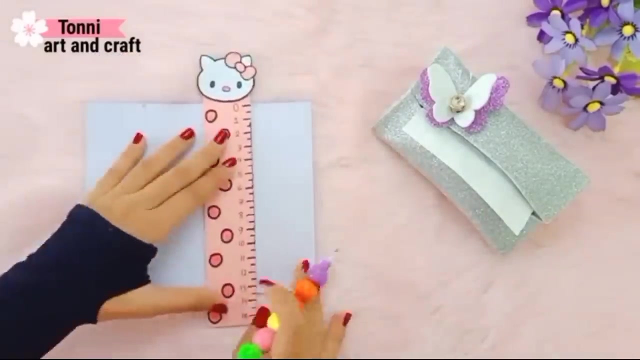 I feel it too, baby, I feel it too, Come around to me. I will hide that you stay close to me all the night, like: Ooh, yeah, yeah, ooh, yeah, yeah, Come around to me. I will hide that you stay close to me all the night, like: 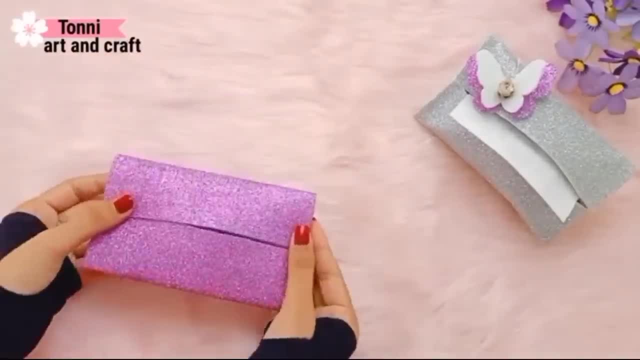 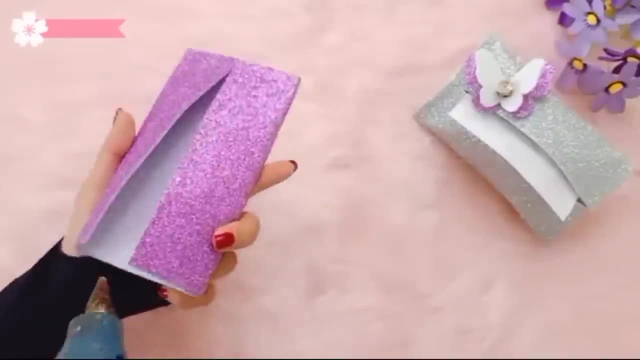 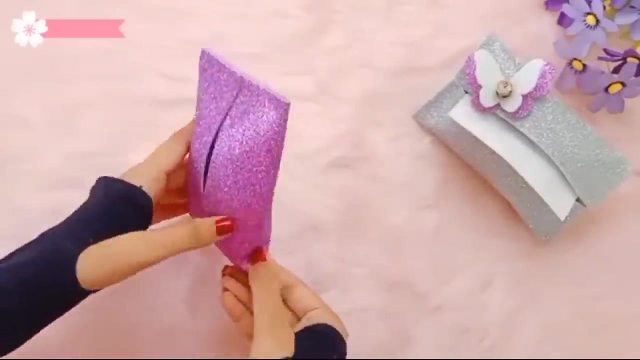 Ooh, yeah, yeah, ooh, oh. I've been thinking of you ever again. Tell me you do, tell me you do. Don't you feel you miss me and you wanna kiss me? I feel it too, baby, I feel it too. 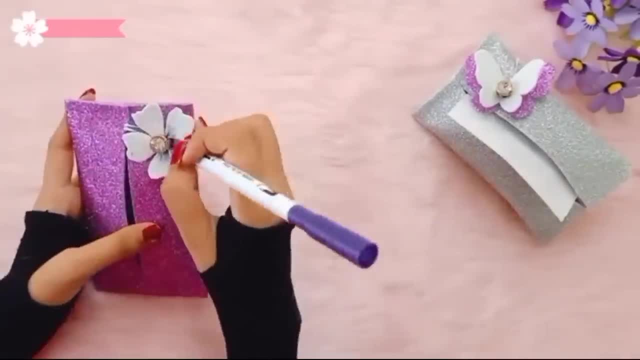 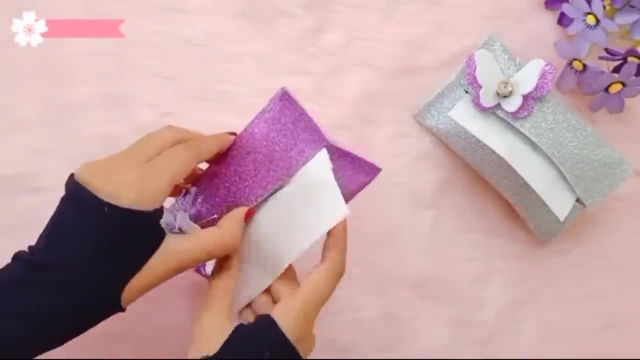 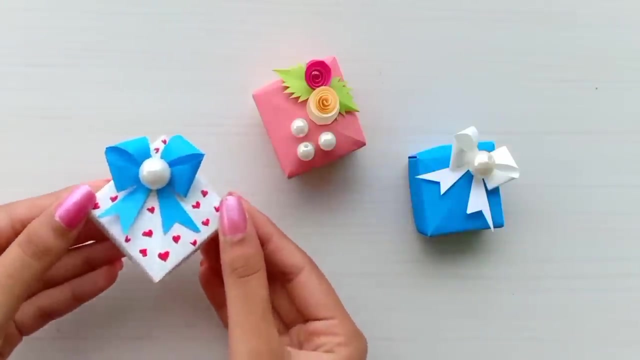 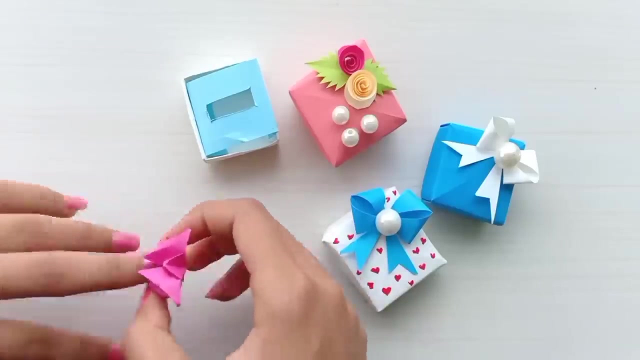 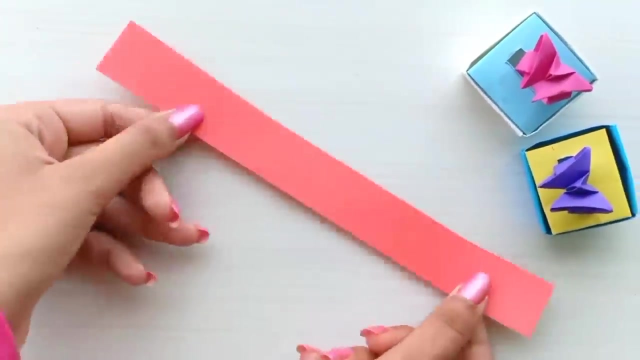 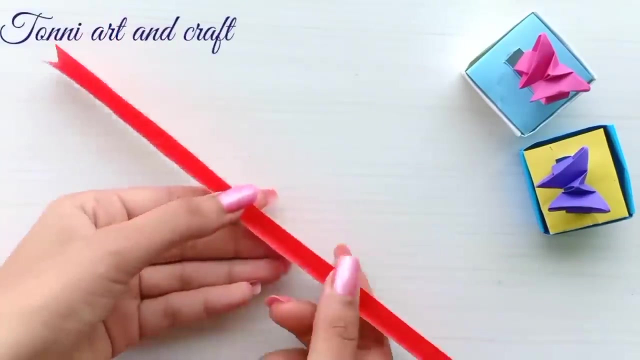 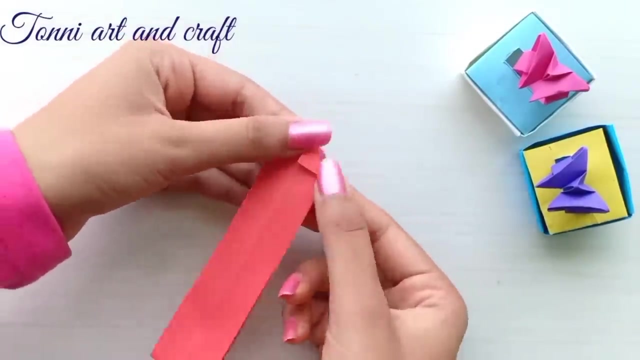 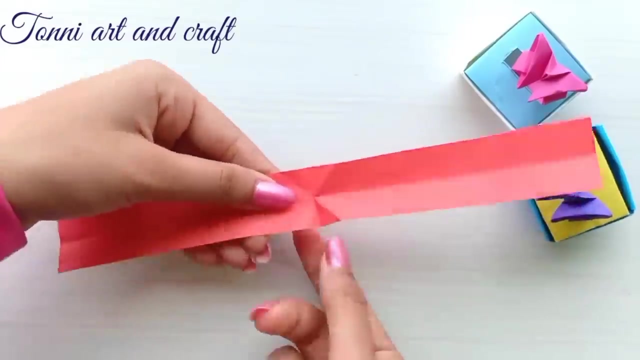 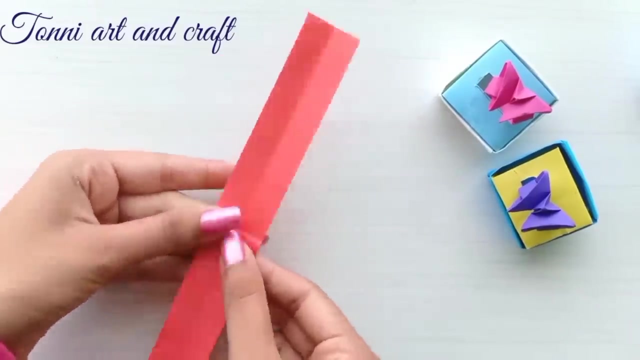 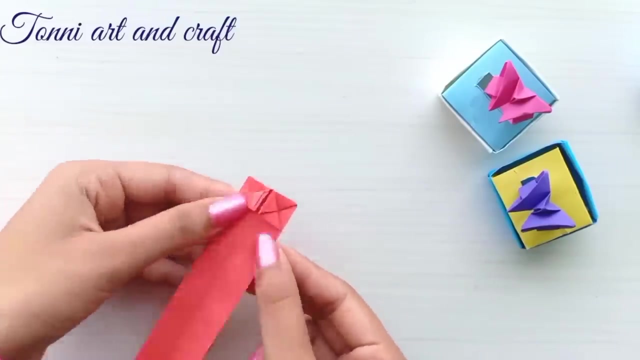 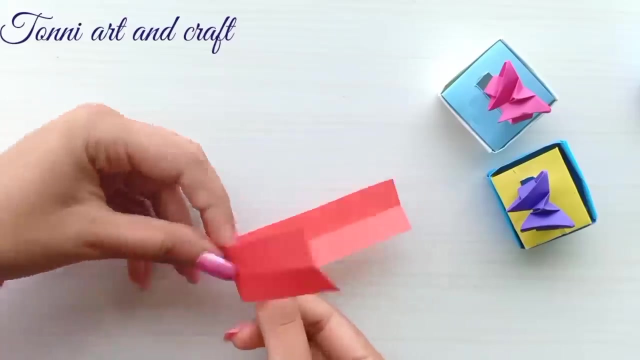 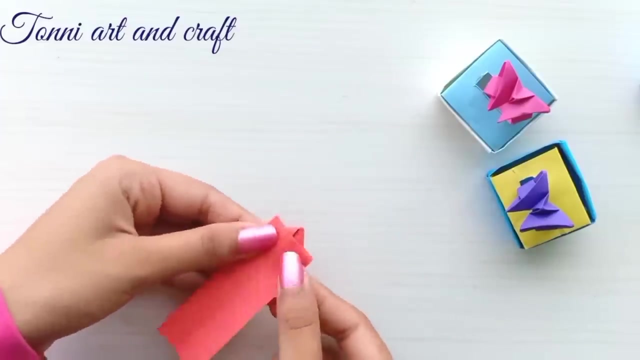 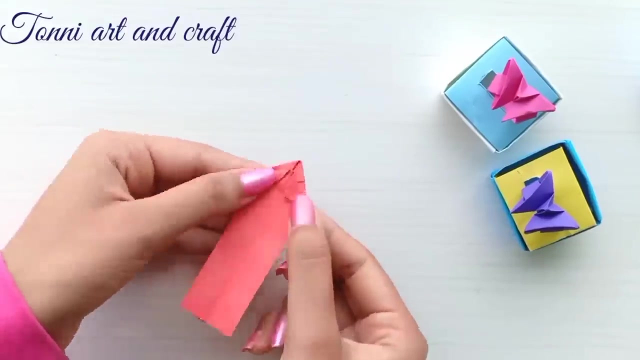 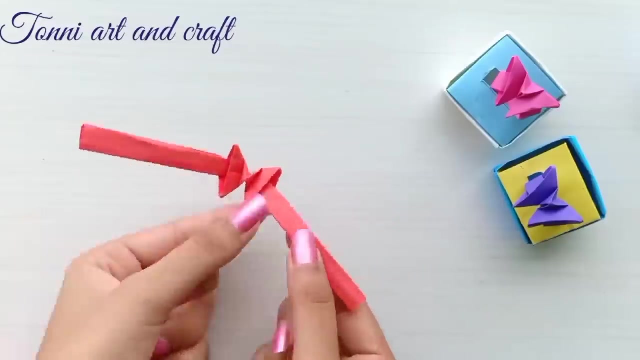 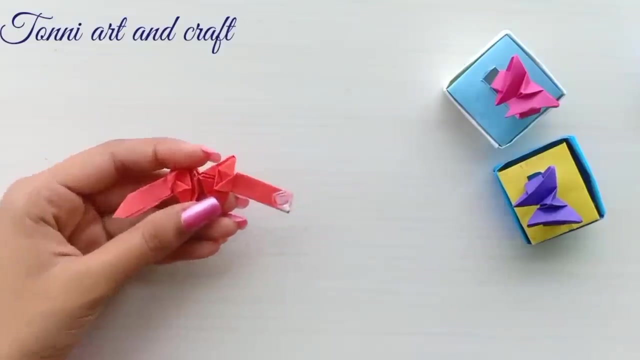 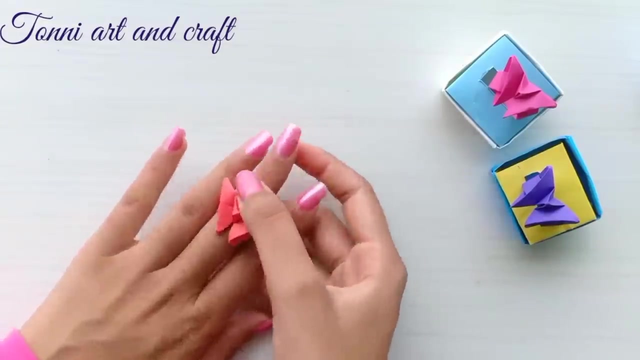 I'll spend the night with you, all the night like Ooh yeah, uh-uh, ooh. I feel it too, baby, I feel it too, Don't you feel it too? ёт mathematics. Thank you, Thank you, Thank you.